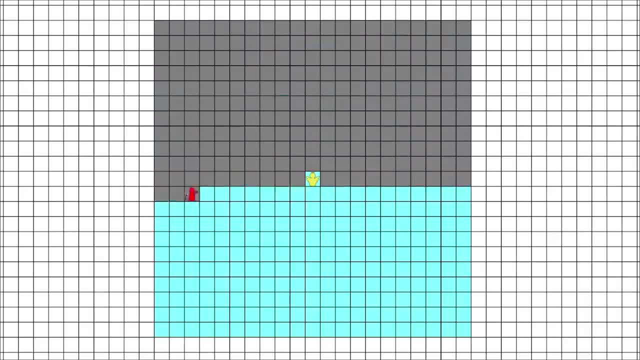 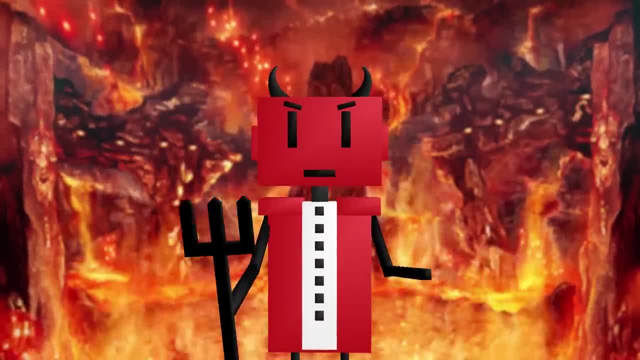 And the devil can only block one square at a time. How can the devil ever have enough time to trap the angel? But today I'll be the devil's advocate. Let's look at the angel's movements a little closer, with a game theory perspective. 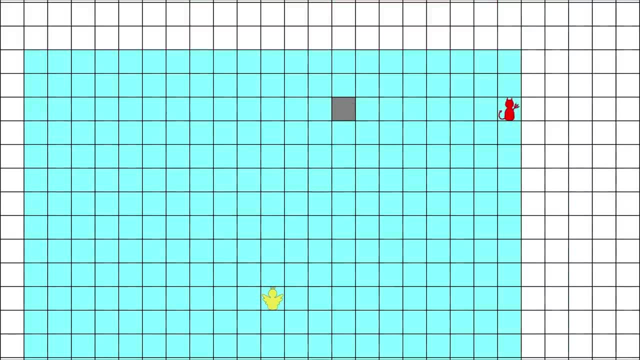 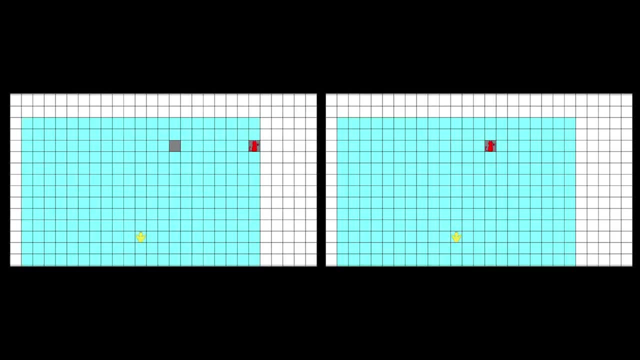 One thing to notice is that the angel would never want to move to a space that she could have landed on previously. The proof is simple: If she took more than one turn to get to a spot that she could have reached before, then the result would be exactly the same. 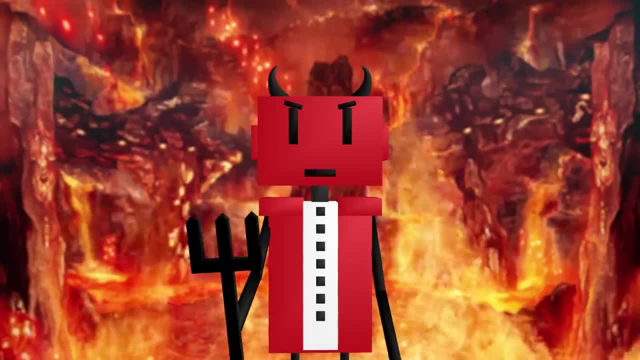 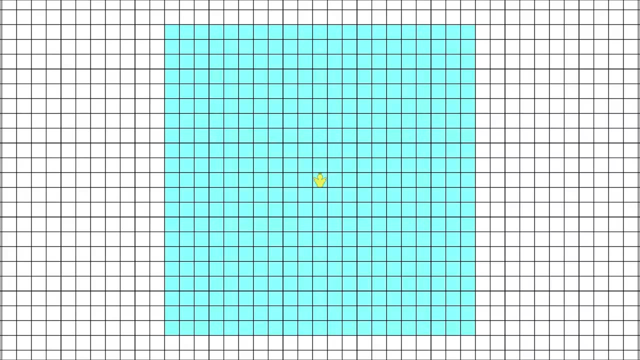 but the devil got extra moves in between. So it's impossible for the strategy to ever help the angel. It strictly benefits the devil. That means all these spaces in between are effectively gone. In fact it can be treated the same as if the devil himself blocked all of those squares. 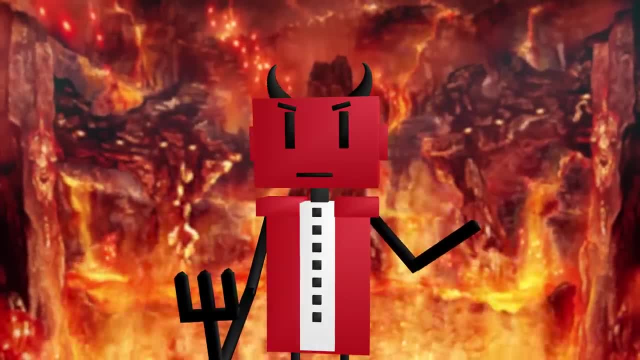 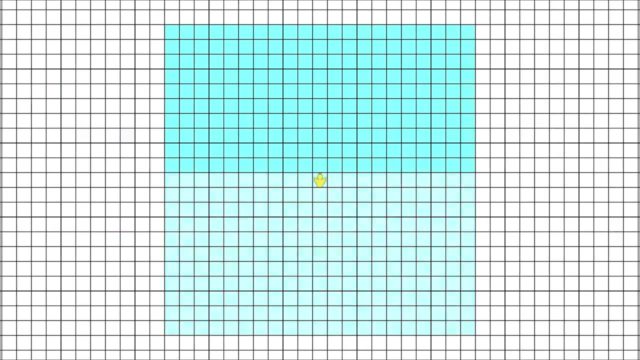 So, even though the devil only blocks one square each turn, the angel blocks a hundred. But that's no problem, we can just keep moving away. right, Let's suppose we restrict our movement to always be some amount north. Well, the devil has a plan for us. 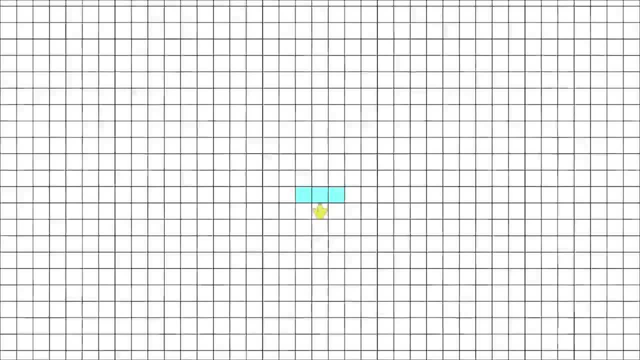 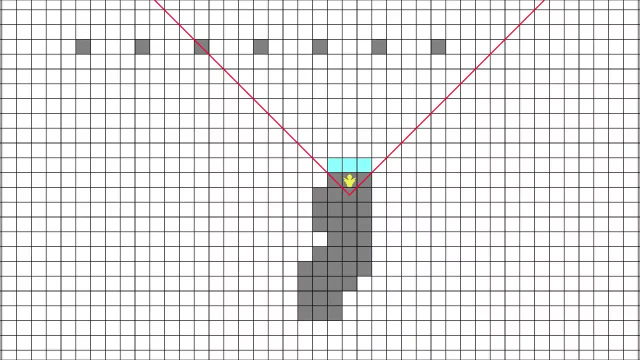 I'm going to switch to k equals one to make the visuals easier. but far away, the devil can start building a wall above our cone of movement, leaving big gaps. Once the angel gets halfway there, the problem recurses as he fills in the next squares. 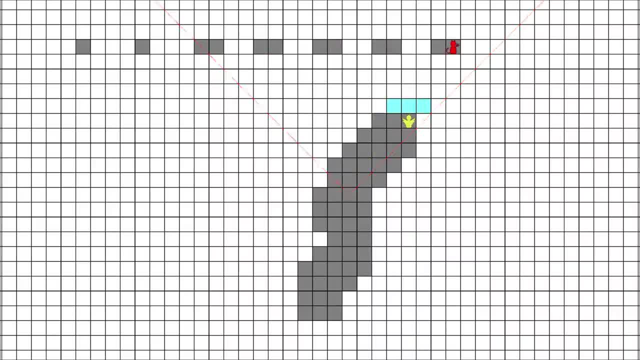 The devil is half the time, but also half the distance, so he can do it. This keeps repeating until the wall is entirely dense and the angel can't move north anymore. This works with any k, but the required distance away to build the wall increases super exponentially. 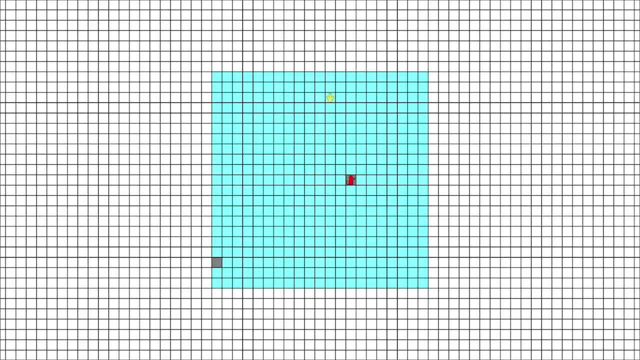 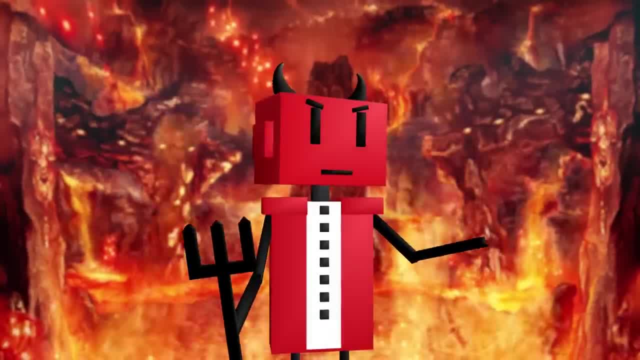 Okay. well, maybe saying we had to move north was too restrictive. I mean, we have way more maneuverability after all, right? Well, Conway also showed that an angel that strictly increases her distance from the origin can also be trapped, using a very similar argument. 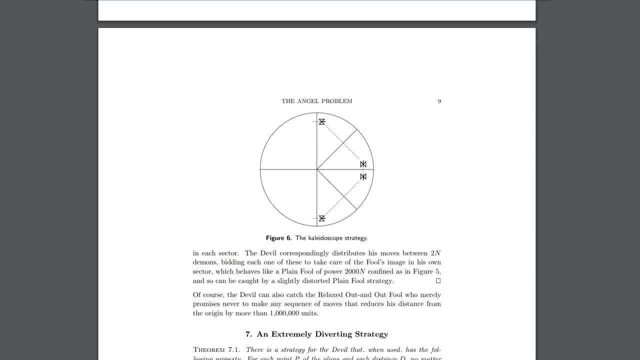 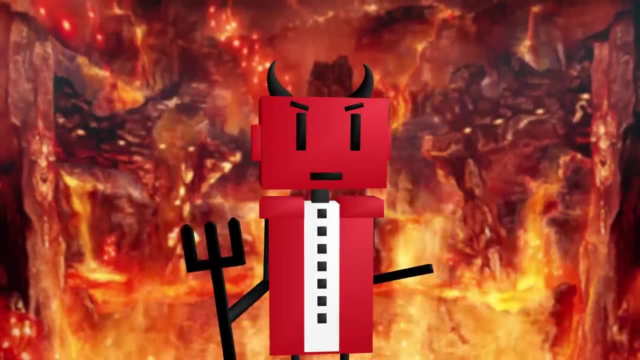 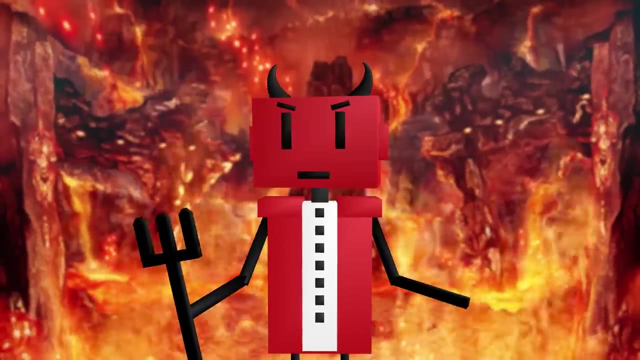 The devil can pretend the angel has a k four times larger and use alternating turns to build walls on all four sides. So have I convinced you? Is there any hope for the angel? Are you willing to sell your soul to the devil? Well, this was an open problem in mathematics.